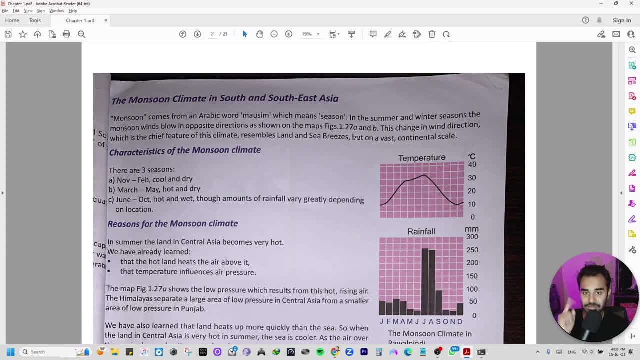 come in my 12th grade, right, yeah, i've just completed my 11th grade, uh, so we were living in ipo, it's like, uh, some a little bit far away from kuala lumpur, the capital kl in malaysia. so the the thing that i noticed over there was, you know, the rainfalls were, like you know, literally. 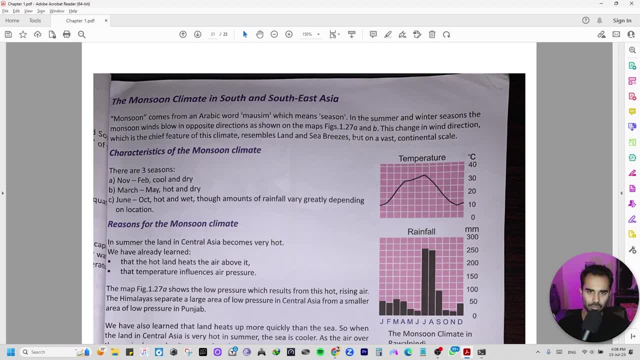 the, the, the clouds were like pouring so much over there, like after every. i mean, like you know, it was so spontaneous over there that in the morning i'm gonna wake up. it's gonna be a shiny, sunny day with a blue, beautiful blue sky. all of a sudden, at 1 pm, 11 pm or something like that, the clouds are. 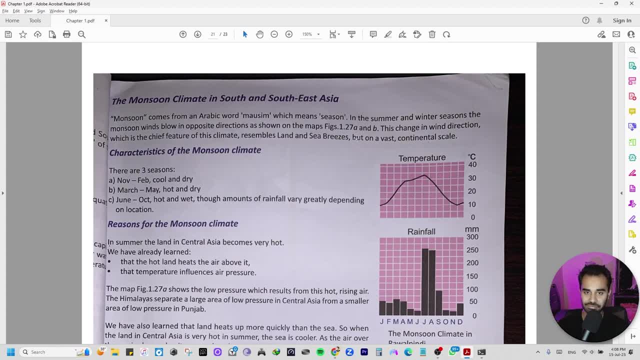 gonna come from nowhere and it's gonna, like you know, be cats and dogs everywhere. literally, it used to rain like that and it was really beautiful. actually, you know, some people like rain, some people don't like rain, but i'm of a thought that i do like rain a lot. yeah, so it says over here. 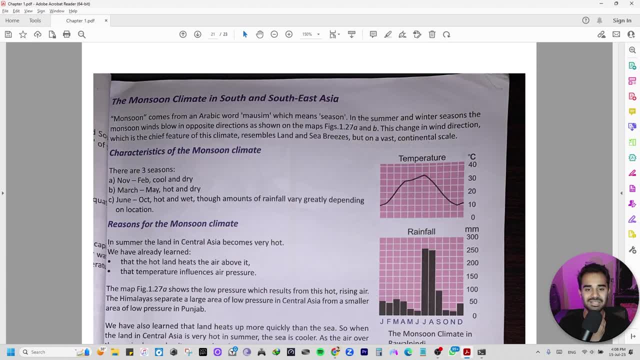 that the monsoon comes with an arabic word, mossim, which means the season in the summer and the winter seasons. the monsoon winds blow in the opposite direction, as shown in the map in figure 1.27 a and b. this changes in the wind direction, which is the chief feature of the climate and resembles the 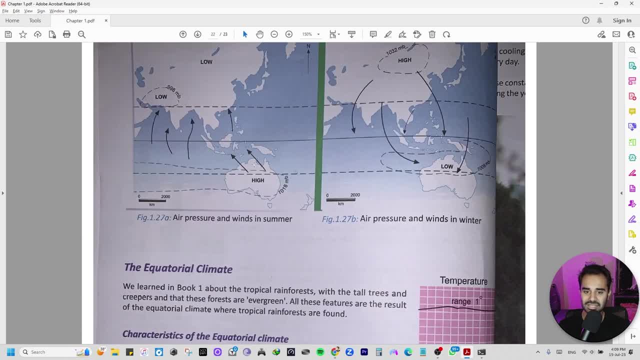 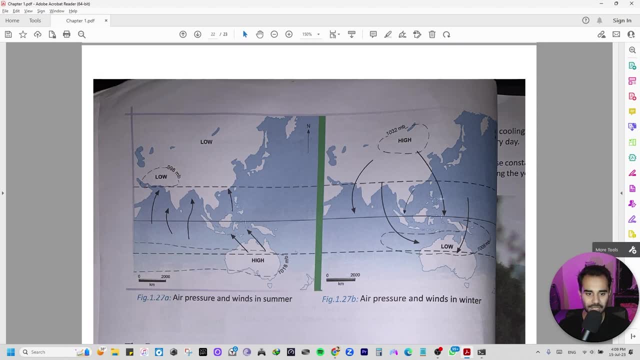 land and sea breeze, but not a vast continental scale. so this is the picture: 1.20, 1.27 a and 1.27 b. so they're showing the southeast asia over here. okay, in the birth pictures they're saying this thing: the air pressure and the winds. in summer they travel from the southern region to the northern. 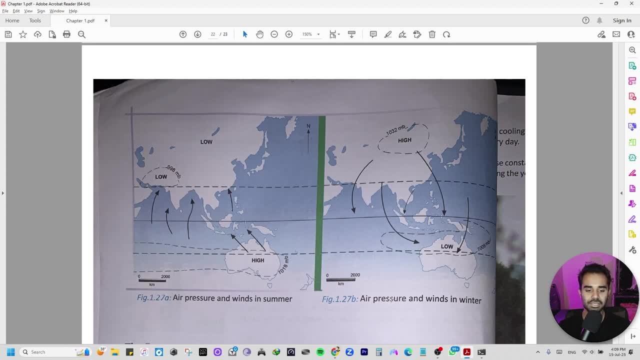 region and speaking about the, the pressure, the air pressure and the winds in the winter. so they're saying the air pressure and the winds in summer. they travel from the southern region to the southern region. all right, so, yep, that was about it. and then it says over here that the characteristics 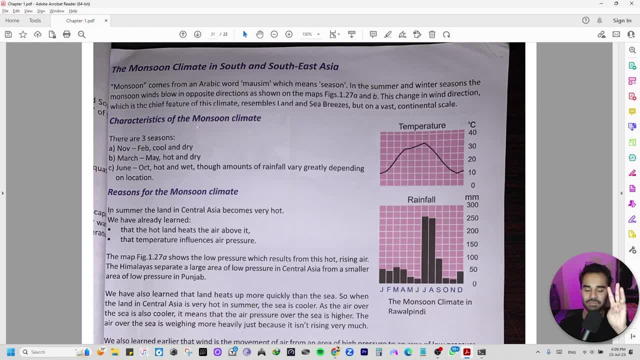 of the monsoon climate. now, what are the characteristics of this monsoon climate? it says over here that we have three seasons. okay, from november to february it's cool and dry. from march to may, it's hot and dry. from june to october, it's hot and wait to uh, though the mountain. that though. 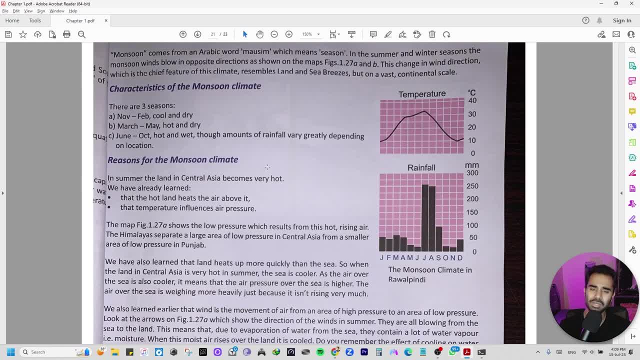 the amounts of rainfall vary greatly depending on the location. yeah, that's true, it really depends on the location.